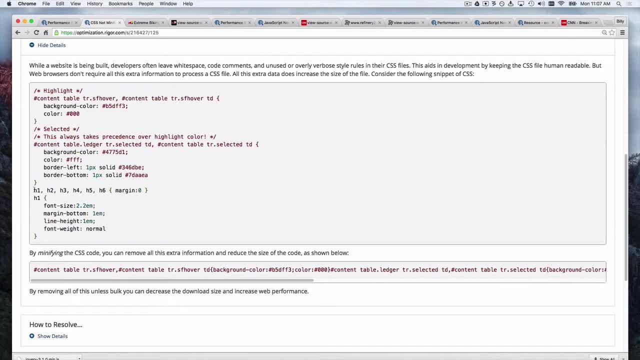 Just discard it. What the browser cares about is knowing that you know the H1 tag needs to be drawn at this font size, And so what minification is? it's about removing white space and comments and things like that, And so you get a nice streamlined thing down here of what the browser 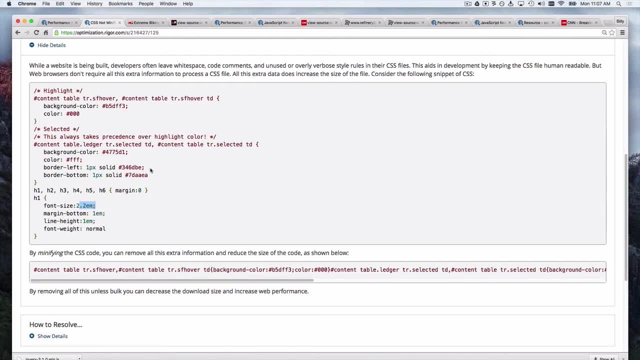 actually cares about. Also, if say, with CSS you could remove unused rules, With JavaScript you could rename the variable names of local variables in a function. All of these things lead to a smaller amount of content, but the same, it means the exact same thing to the browser. 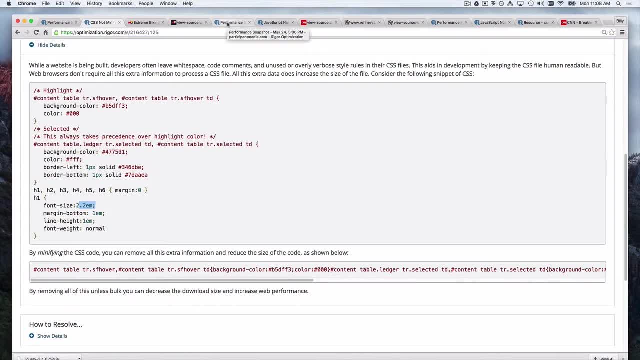 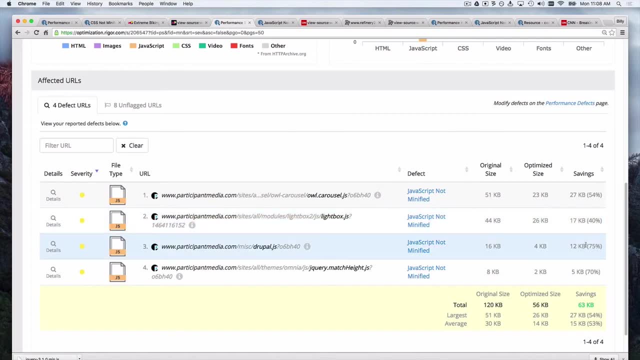 Now, surely that can't be that much savings. I mean some comments and some white space. Well, it turns out it is In this case. we see these four JavaScript files on average could have at least 40% savings. Two of them could have 70% savings, And that's because 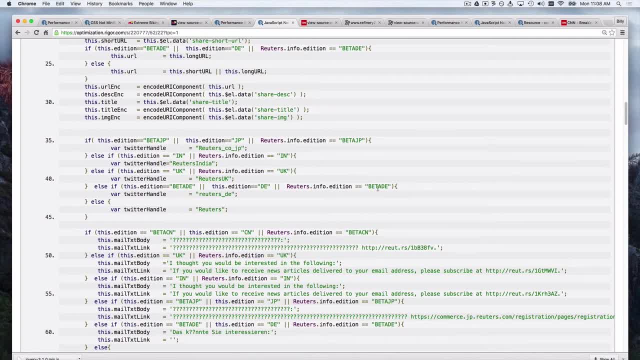 people tend to write code and CSS and things like that with lots of white space. They're thinking about the developers and the human and not really thinking about the browser that's going to render this. Well, you can minify it, And not just CSS and JavaScript. Here's CNN's homepage, the: 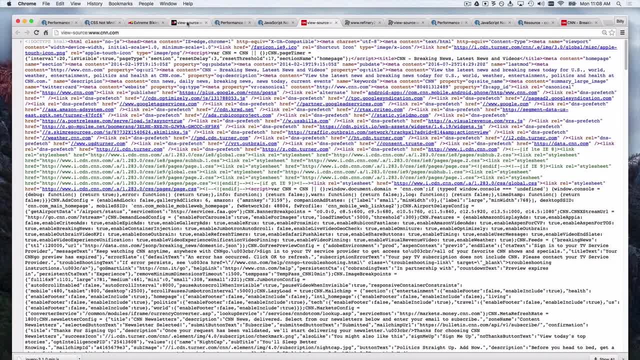 source and we can see they've minified the HTML. It looks very different than the source from Red Bull, So it's actually smaller and can be transmitted faster. Now it's not just your obvious text things like HTML and CSS and JavaScript. Here's actually an SVG image. 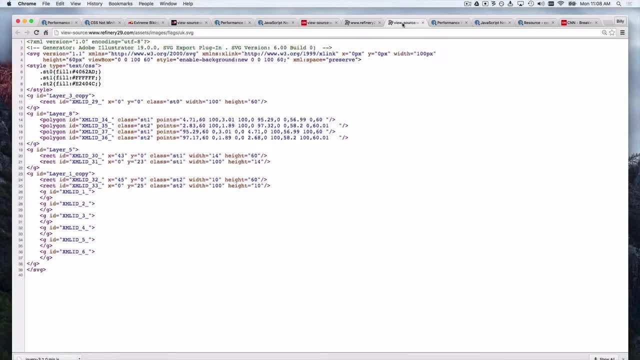 from Refinery29.. Now SVG images. they're just text, So you can minify these the same way you would anything else, You know: remove comments, remove white space, delete comments and ultimately, make the file smaller. Now there's something you should consider when 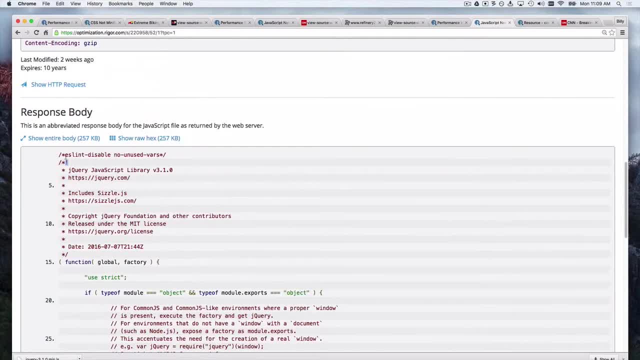 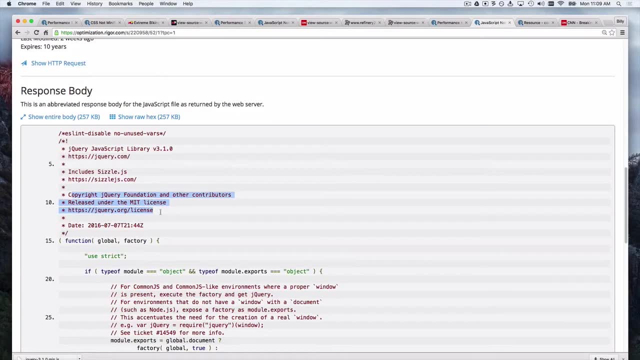 you're actually doing minification, which is that sometimes there are certain comments that can't be removed. So in this case, we actually see here's jQuery And jQuery. it has its licensing information and copyright information in this And if you ran this through, 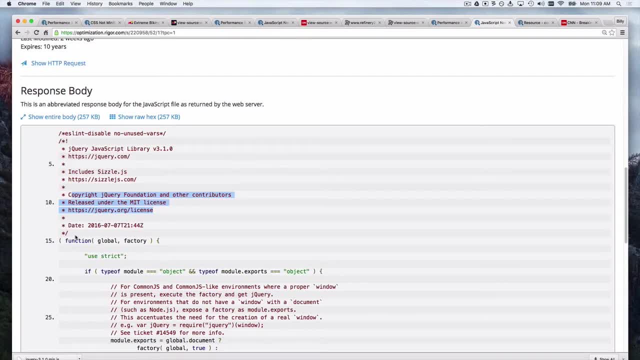 a minifier and it got stripped out. that would suck right, And in fact in many cases that's a violation of the license, And so if there's a comment that you don't want to have removed for legal reasons or whatever, you can just remove it, And then you can actually get a. 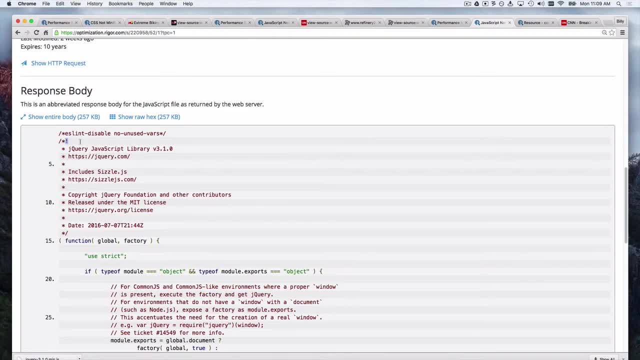 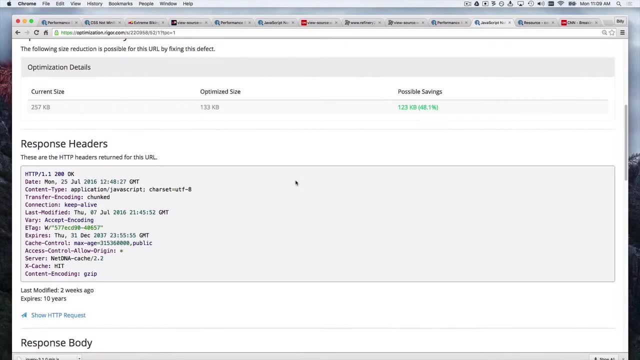 comment And if you're going to do minification, you actually can put an exclamation point at the beginning And all minifiers respect this. This is called an important comment and it won't strip the important comment. Now a lot of people ask: when should I do? 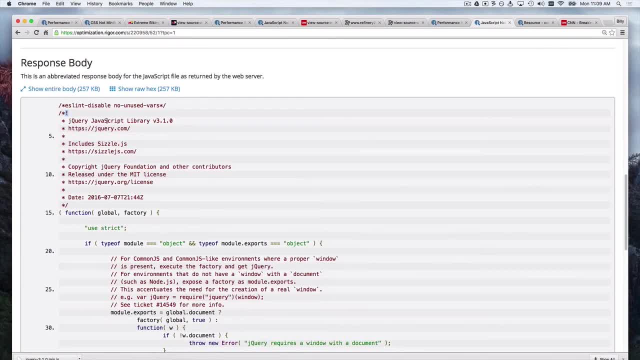 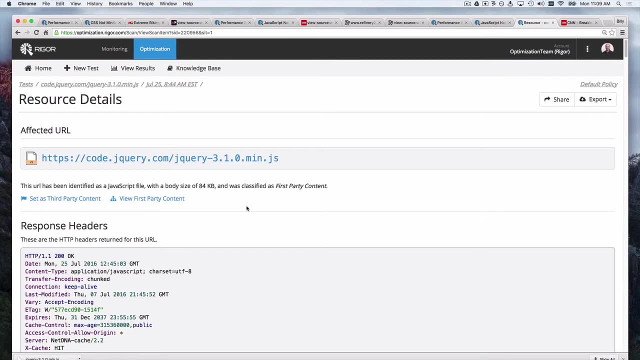 minification. I want to be, you know, working and editing on the great file, not the minified file, And that's totally true. A lot of times, build systems or even editors can be hooked up so that when you save the base file, they'll auto-generate this minified file. So this: 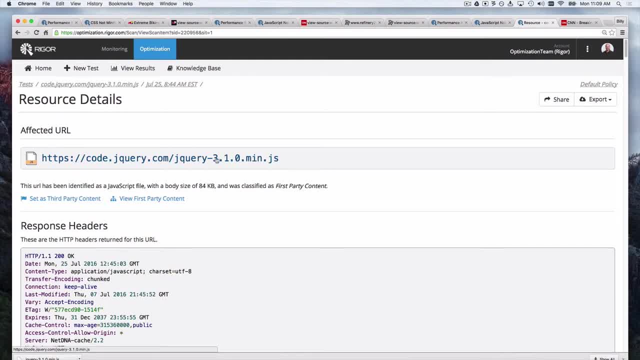 is jQueryminify. You see this naming convention. It's very common And there's tons of different build scripts and publishing pipelines. I guarantee you, whatever's doing your bundling and versioning and all of that stuff, there's a minification object. So take a look Now. some people will. 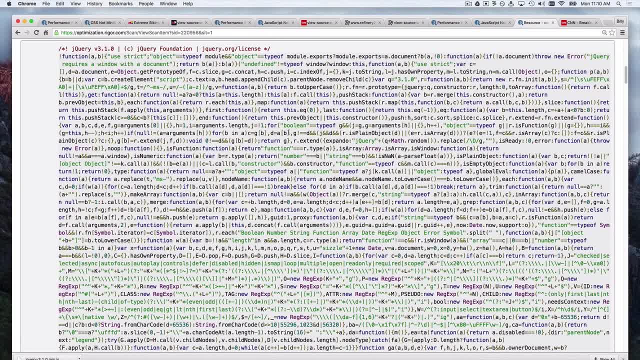 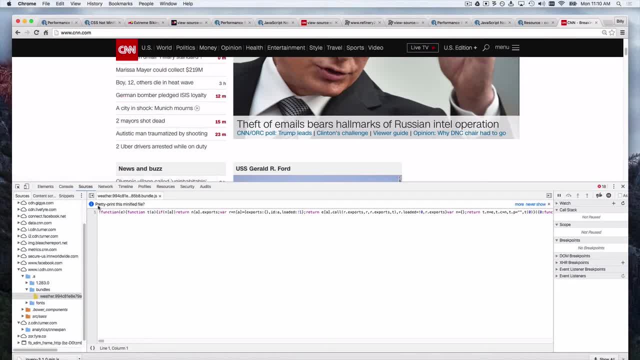 say: well, we're losing something. We're losing the ability to kind of go in there and see what all the really cool stuff is, And that's not entirely true. So here is a JavaScript file from CNN and you can see it's minified all to one line, But all of the browsers have. 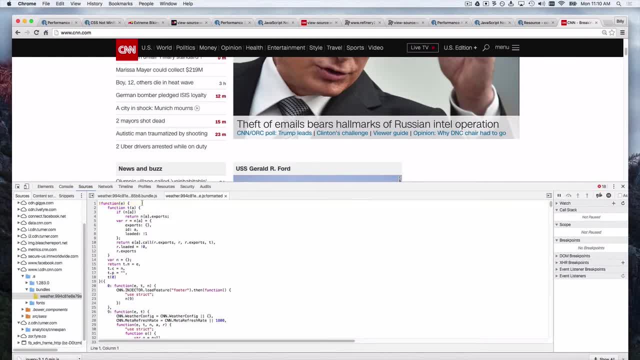 a really cool built-in, pretty printable minifier So we can see what's going on. There are also these things called map files which when you're debugging, kind of translate back lines and offsets in the minified file back to the original file So you can do a better job debugging. 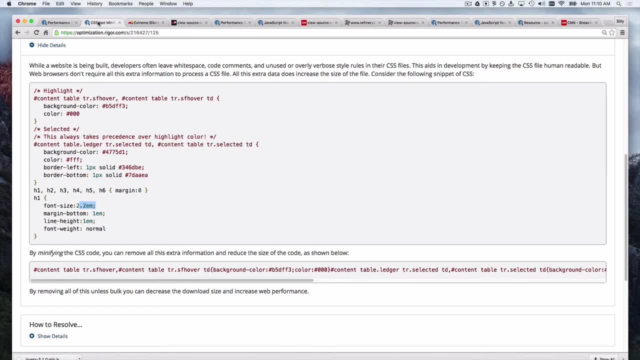 So that's minification. It's really focused on what can we remove that is helpful to a human but is not helpful at all to the browser? to try to reduce the size of our content and ultimately speed up the performance, The performance of our sites.